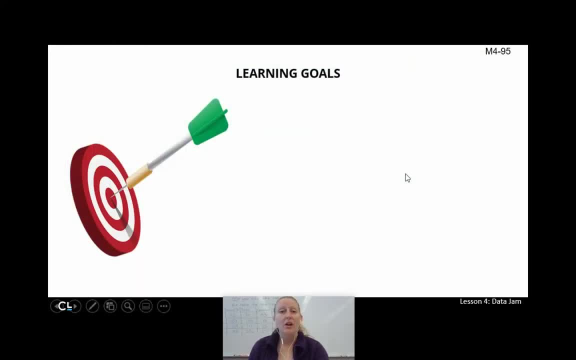 So that's what we're going to be focusing on today. So our learning goals for today and next time. we're going to recognize possible associations and trends in categorical data, right, What's the trend that's happening? We're going to use that categorical data to make decisions, all right. 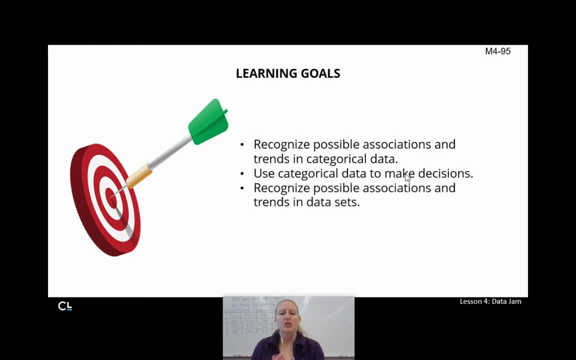 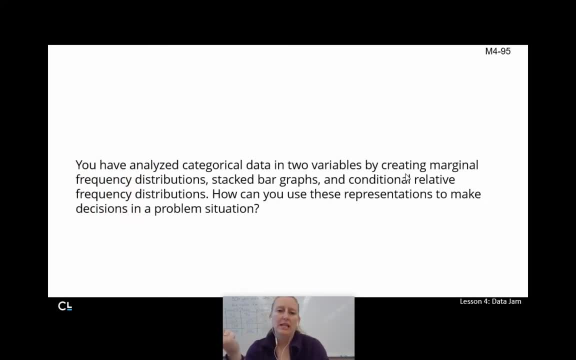 This is the pattern we see. so what decision are we going to make? And also recognize possible associations and trends in data. So you've analyzed categorical data in two variables by creating marginal frequency distributions, stacked bar graphs, conditional relative frequency distributions. we've done so many things. 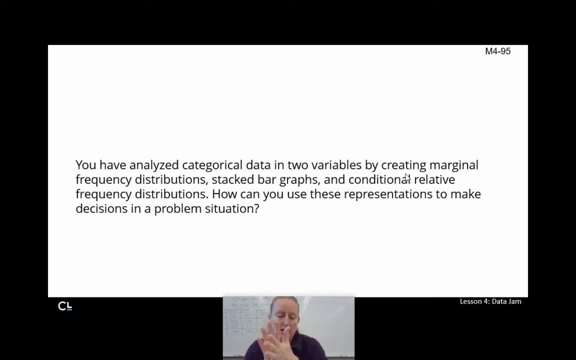 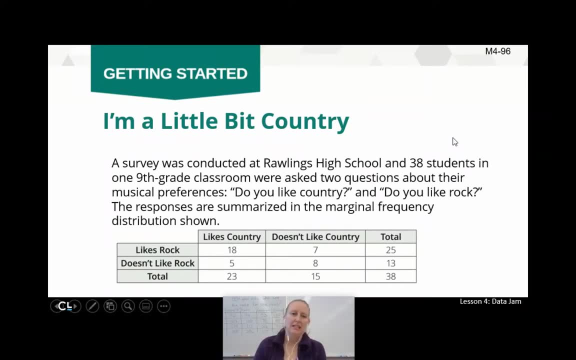 How can you use these representations to make decisions in a problem situation? So, to take it a little further, we're over on page M4-96.. A survey was conducted at Rawlings High School And 38 students in one Ninth grade classroom were asked two questions about their musical preferences. 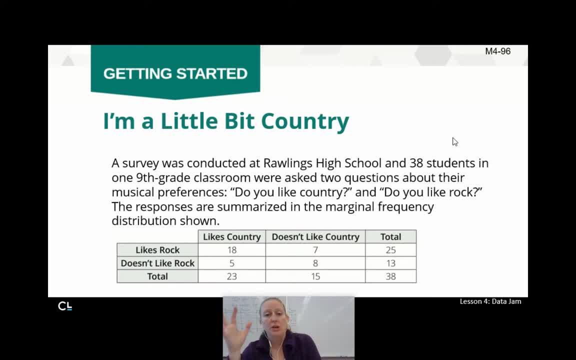 Do you like country, Do you like rock? The responses are summarized in the marginal frequency table. So do you like country? They do or they don't. Do you like rock? They do or they don't. Of course, it's a marginal frequency table, so we have our tables hanging out here as well. 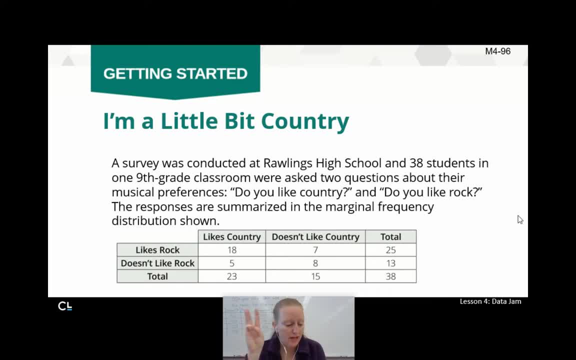 On the page. I've got three questions, Questions one, two and three. They're on page 96.. Go ahead, You might want to have a question. You might want to have a calculator handy. Answer the questions. Hit pause. work this out, hit play when you're ready to check in. 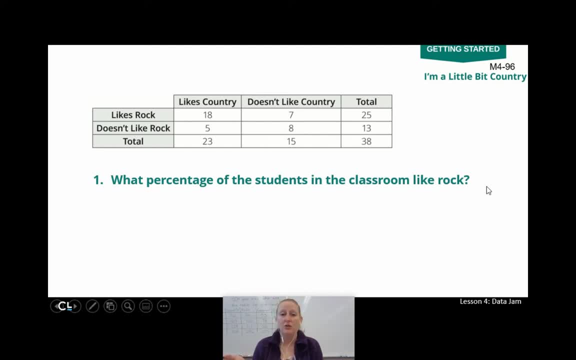 So question number one: What percentage of the students in the classroom like rock? I grabbed my calculator and I was like, okay, 18 students. whoa, I'm trying to think I like rock. I'm trying to think who likes rock. 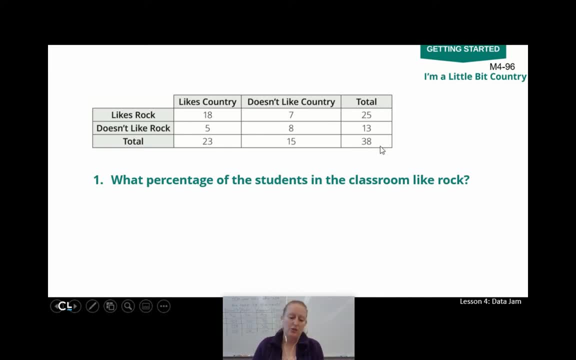 Twenty-five students like rock, So 25 out of 38. So I did 25.. Divided by 38, they want a percent, so I multiplied by 100. And I found I got 65.8% of the students in the classroom like rock. 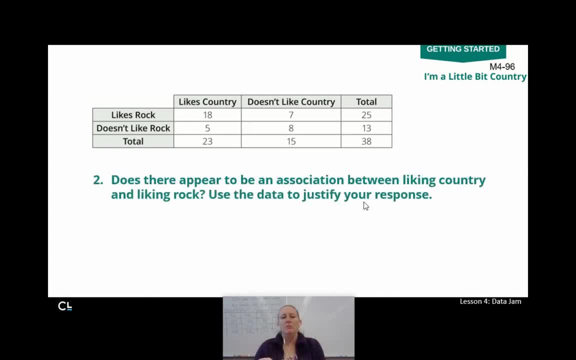 Does there appear to be an association between liking country and liking rock. Well, if they liked country, it does seem that they liked rock. It does appear that there's an association. But if those who like country music, they like rock. If those who like country music, a lot of them like rock music as well. right, 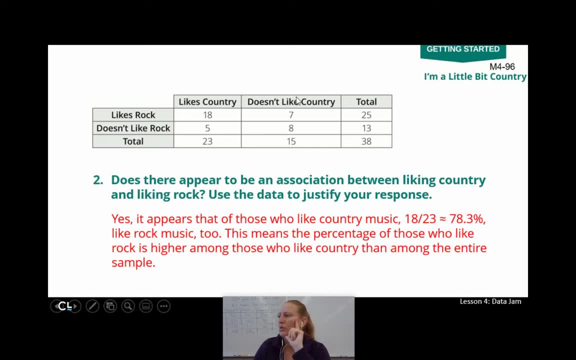 Like country and they like rock, Definitely the biggest out of all four of these numbers here. So this means that the percentage of those who like rock is higher amongst those who like country than amongst the entire sample Right. So 18 out of the 23, that's 78%. 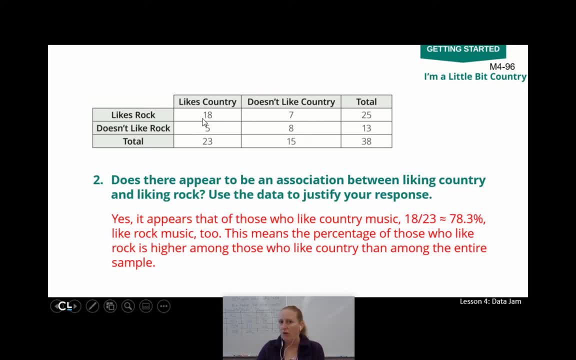 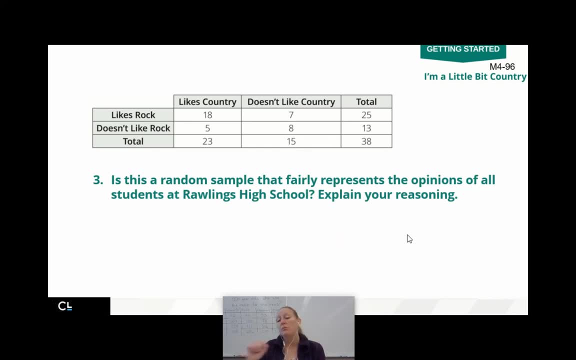 So of the students that like country, 78% of them like rock as well. So definitely some association there. Is this a random sample that fairly represents the opinions of all students at Raleigh High School? Explain your reasoning. I'm going to say it's not a good sample because we only asked ninth graders, right? 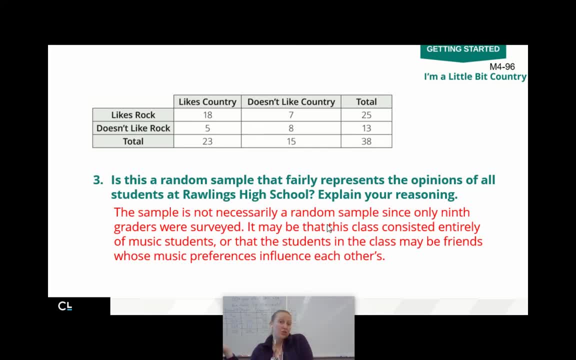 We asked one class of ninth graders. It may be that other grades feel differently, right, It may be this class was entirely music students. It might be that the students in this class were all friends And so they all like the same stuff. 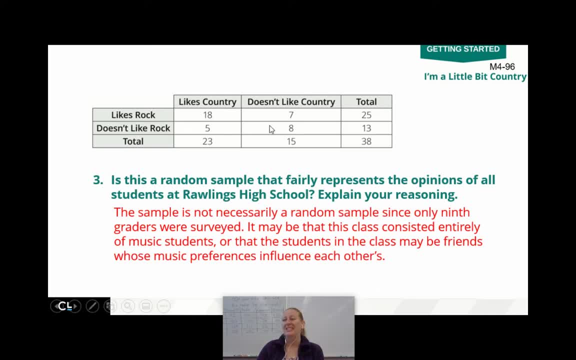 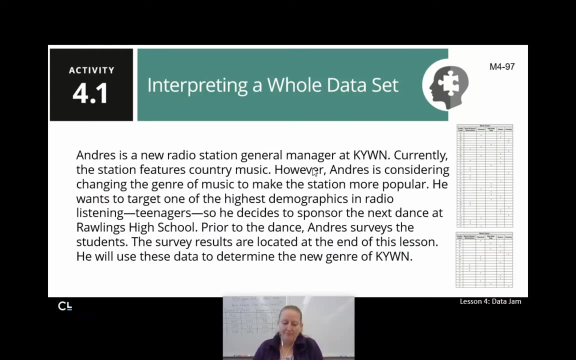 Right. So I don't feel like this is a very good sample of everybody's opinion of the high school. I feel like I would need to ask that the classes get other grades involved. So page 97.. Andres is a new radio station. general manager at KYWN. 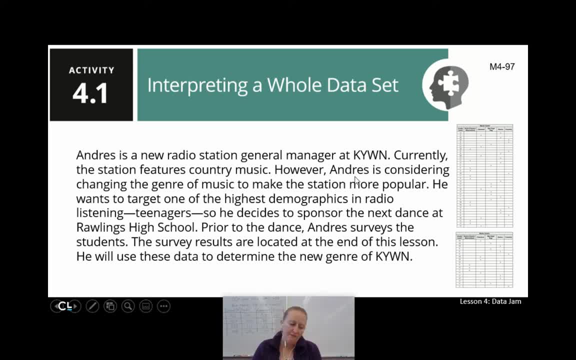 Currently the station features four students. Currently the station features country music. However, Andres is considering changing the genre of music to make the station more popular. He wants to target one of the highest demographics in radio listening and that is teenagers. So he decides to sponsor the next dance at Raleigh High School. 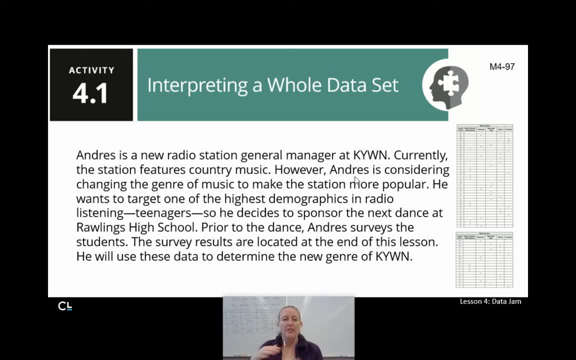 And prior to the dance: Andres surveys the students And the survey results are located at the end of the lesson. So if you're not sure where the survey results are, because this is so tiny on my screen, it's really hard to read. 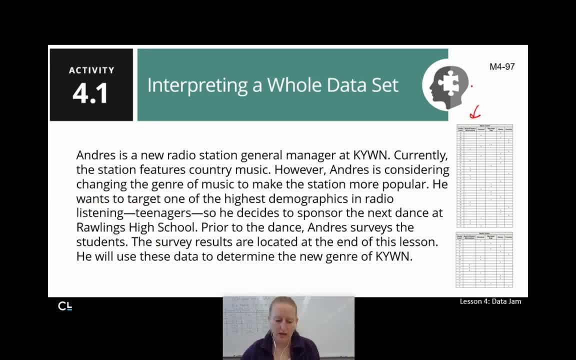 So if you're not sure where the survey results are, I'm going to point out These are on page 4101,, if you want to flip over and take a look, And also 102, because it was a really, really big table. 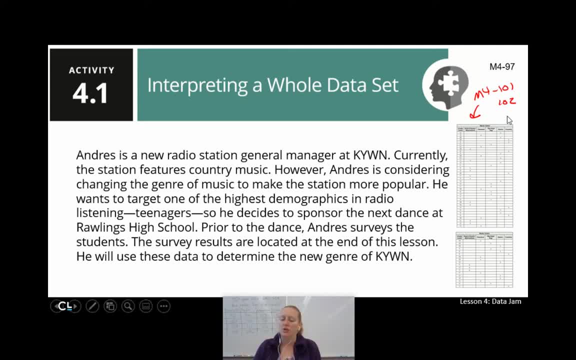 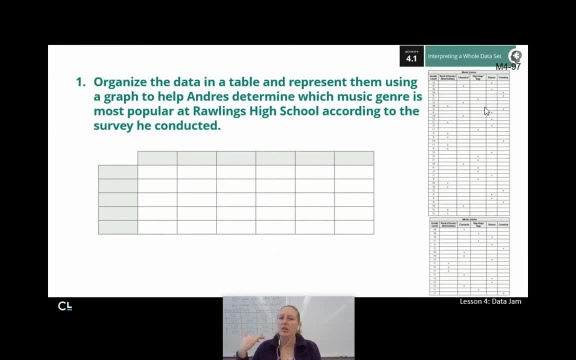 So the survey results are over on these pages over here, because I can't really fit them on my screen very well. So you're going to want to flip back and forth a little bit And, just to start, I want you to organize the data in a table and then represent it using a graph. 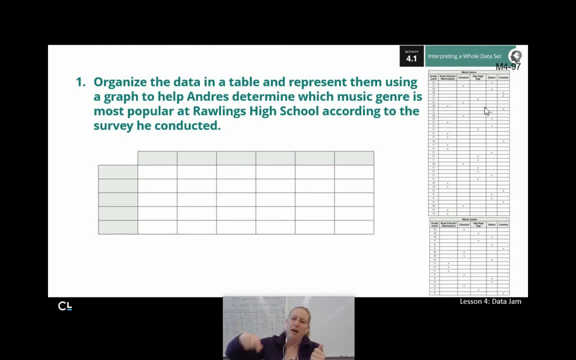 So just start with the marginal frequency distribution table, Make sure you label the top, label the side, Do your tally marks, all that good stuff, And then make a table out of it. So hit pause, Work this out, Get the player ready to check your rank. 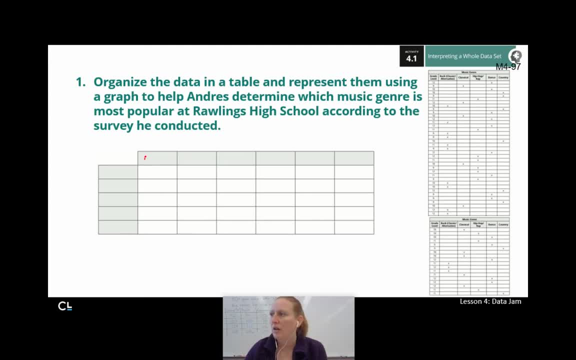 To start, I'm going to label my stuff. So this was rock, This was classical, This was hip hop or rap. Over here I've got dance, I've got country And then I've got my totals. So this is my favorite music genre. 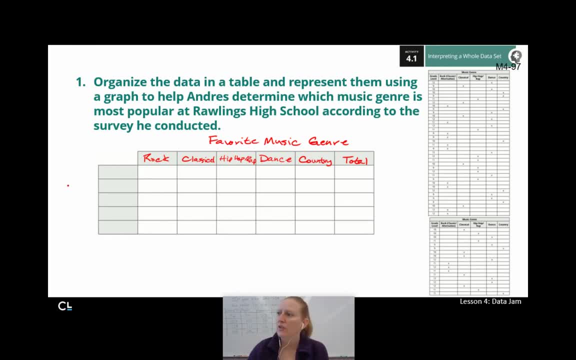 And then down the side, of course, I'm going to do my grade levels, Grade Oh, wow, That's original. So down the side, I've got my grade level, And so we had, of course, high school. 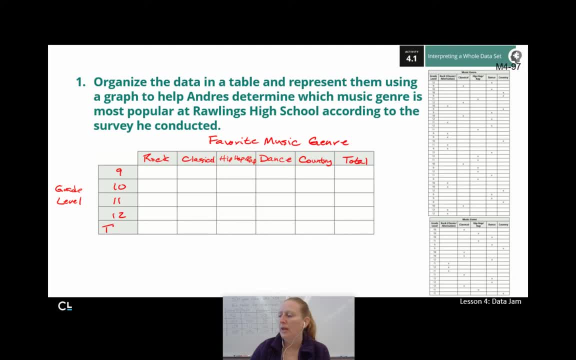 So we had 9th grade, 10th grade, 11th grade, 12th grade, And then, of course, we have our totals. So at this point I hope you went through, I hope you made all the tally marks. 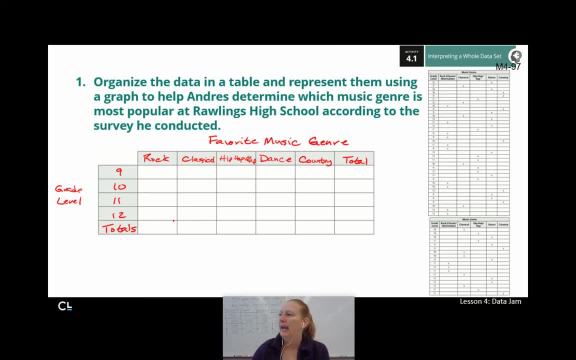 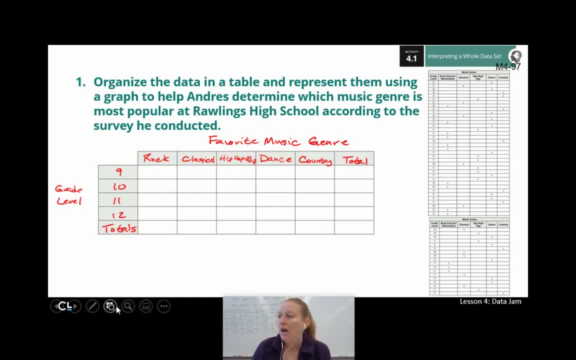 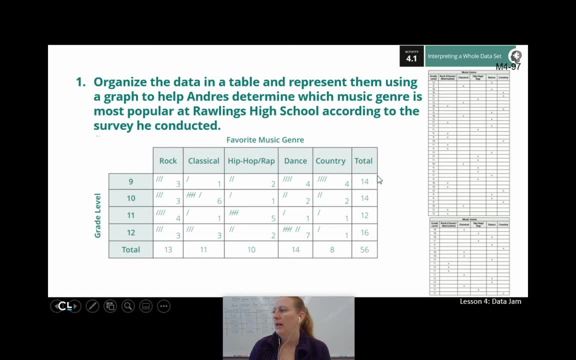 I'm not going to go through the process here because I presume you already did that. I am, however, going to erase this and bring it up There. we go, Bring this up. So 3, 1,, 2,, 4,, 4,, which added up to 14.. 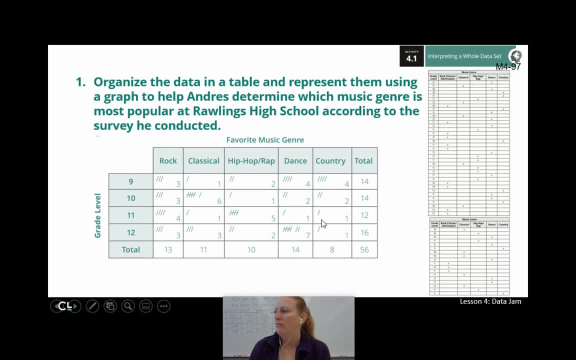 3, 6, 1, 2, 2,, which added up to 14.. 4, 1, 5, 1, 1,, which added up to 12.. 3,, 3,, 2, 7, 1, 1.. 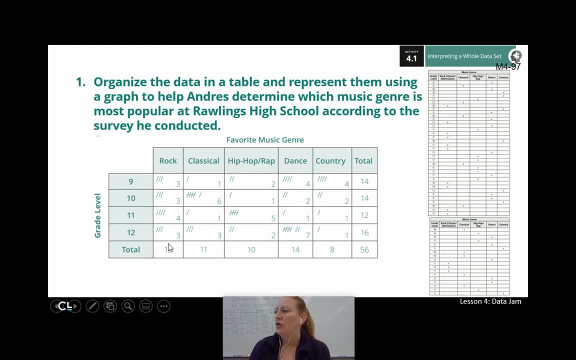 2, 2,, 7, 1,, which added up to 16.. So the total for rock was 13.. The total for classical was 11.. The total for hip hop and rap was 10.. The dance total was 14.. 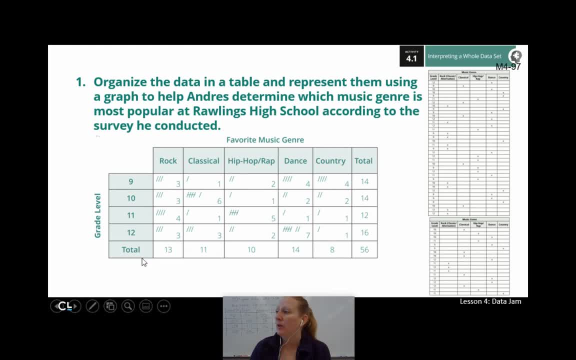 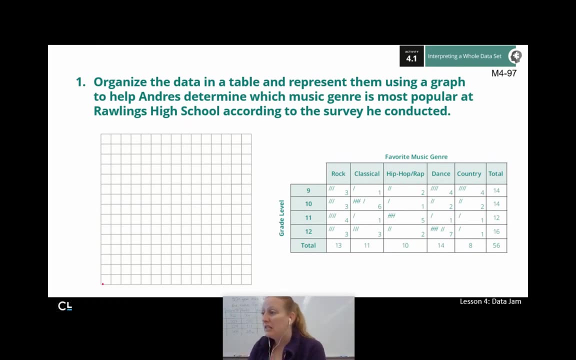 The country total was 8. And my overall total- whether I added it by grades or added it by music- overall total was 56,, which feels a little low. I feel like they should have been a bit more than that. I'm going to go ahead and do a stacked bar graph for this, just to make my life a little bit easier. 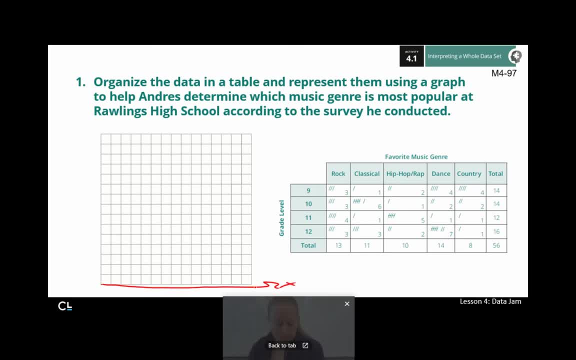 So I'm going to do a stacked bar graph. I'm going to say my x-axis, I'm going to say that's my music, And then for my y-axis, I'm going to say that's the number of students, And I'm going to do a stacked bar graph, even though these aren't percents. 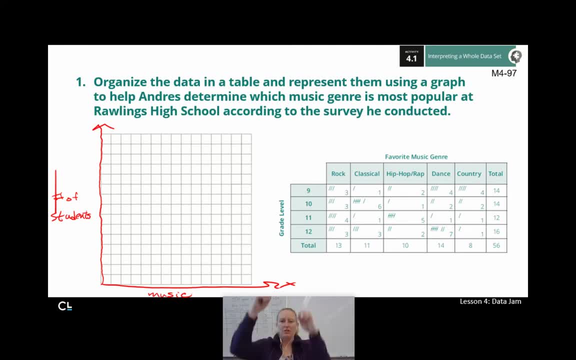 I'm going to do a stacked bar graph just so I don't have like a million bars. It makes it a little easier that way. The biggest number is obviously 56.. It's the biggest, But other than that, the biggest number I see here is 16.. 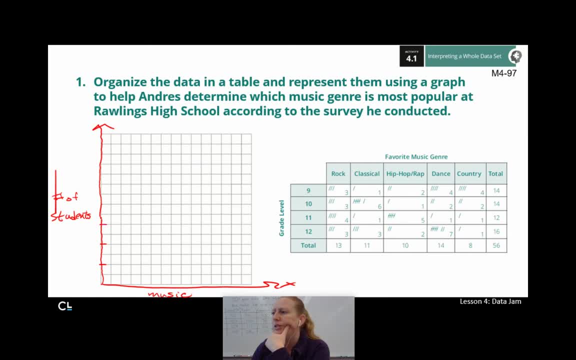 So I think I have enough right If I do 2,, 4,, 6,, 8,, 10, 12.. Maybe I know, if I have enough, All right. So let's do 4,, 6,, 8,, 10,, 12,, 14.. 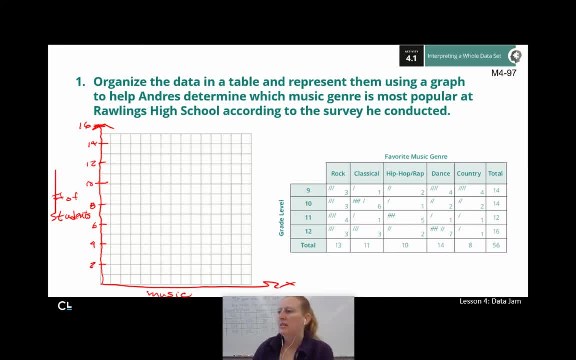 I guess up here will be 16.. So go a little bit off track. But it's not the end of the world. Again, we do need to make a key. So I'm going to go ahead and make a key for each grade level. 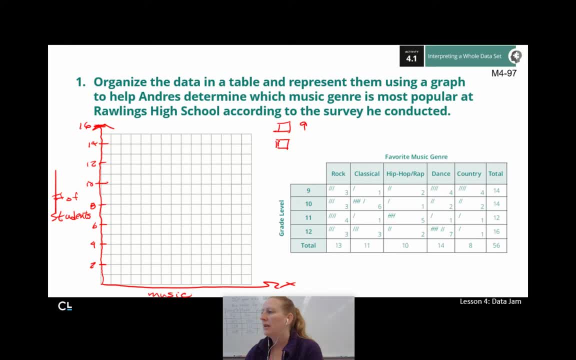 I'm going to say that my empty box is my 9th graders. I'm going to say that my colored in box is my 10th graders. I'm going to say that my- I don't know- vertical stripeys are my 11th graders. 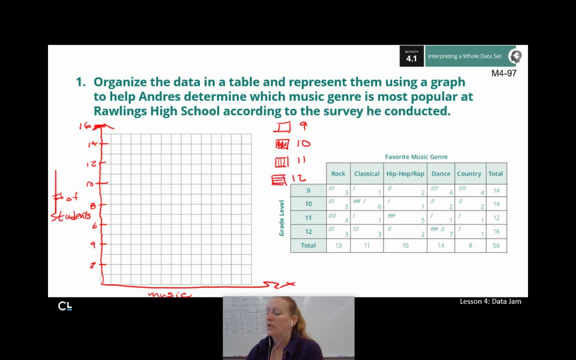 And I'm going to say that my horizontal stripeys are my 12th graders. You can use different colors And of course, you can also use different colors. So for let's see, so for rock. So I've got my 9th, 10th. 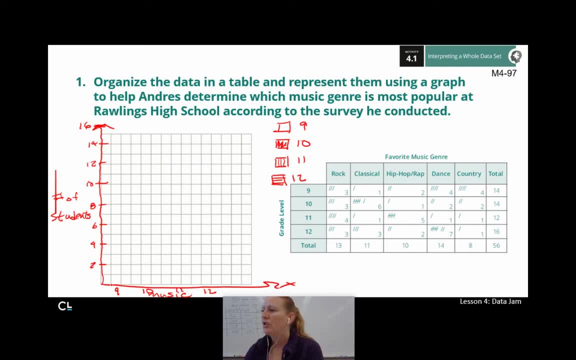 Big space in between here, 11th and 12th, All right. So for my 9th graders, it looks like I've got to go up to three of them that like rock, My empty one. Three 10th graders that like that like rock. 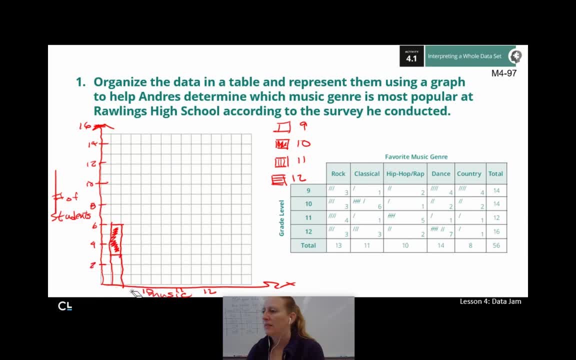 I did this wrong, Missed that. What are you doing? You know what I did wrong, don't you? This should be rock, This is rock. Yay, So three 10th graders that like rock, Four 11th graders. 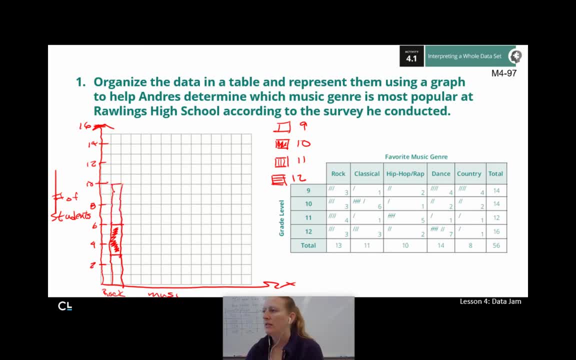 One, two, three, four. So that's going to be my horizontal stripeys, And then three 12th graders. So one, two, three, two, two, And that's not in vertical. My horizontal stripeys are: those are vertical stripeys. 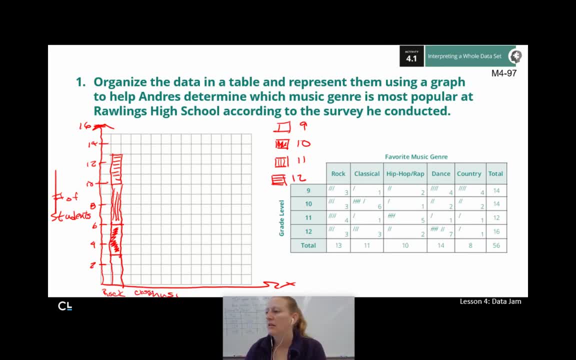 Next up, I've got classical. So my classical, let's see, I've got one 9th grader. I've got six 10th graders: One, two, three, four, five, six. I have one 11th grader with my vertical stripeys. 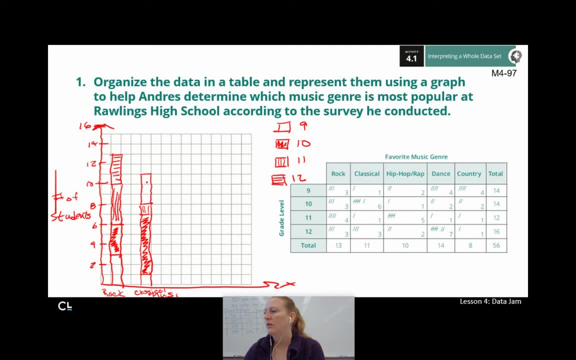 And I've got three 12th graders with my horizontal stripeys. Hip hop is next Hip hop and rap. And I've got two 9th graders, One 10th grader, Five, one, oh dear. 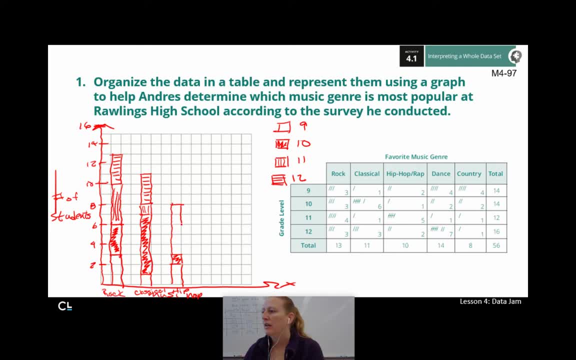 Five: one, two, three, four, five 11th graders with my horizontal stripeys And two 12th graders. Sorry, those are vertical stripeys, My horizontal stripeys. Oh, they're terrible. Next up, I've got dance. 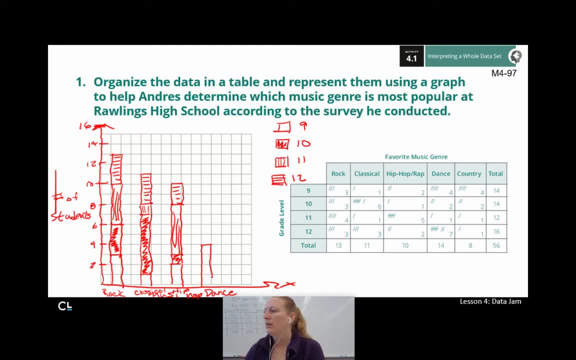 So for dance, I've got four 9th graders: One, two, three, four. I've got two 10th graders, One, two. I've got one 11th grader with my vertical stripeys. 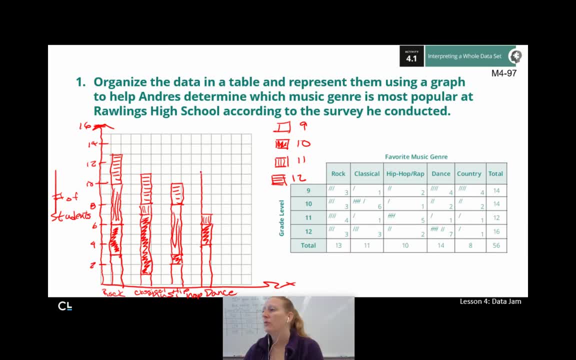 And seven 12th graders: One, two, three, four, five, six, seven 12th graders. Wow, With my horizontal stripeys. Last but not least, we have country With four 9th graders. 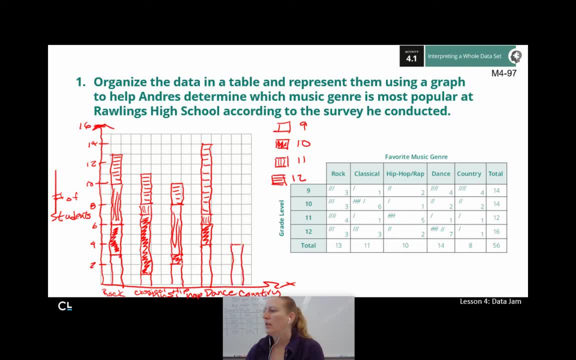 So three, four, Two 10th graders, One 11th grader with vertical stripeys And one 12th grader with horizontal stripeys. So this isn't the prettiest thing ever, but it fits on my graph. 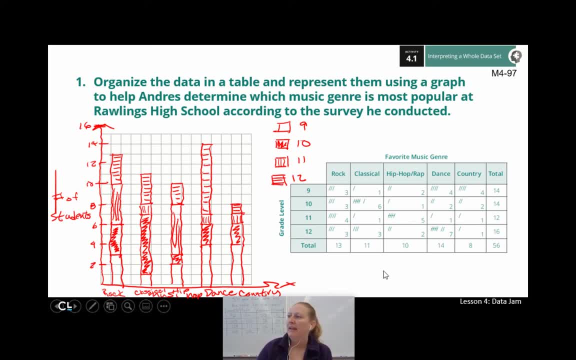 It does a pretty decent job of things, I reckon Definitely gives me a good feel. for who liked what, I will say that, Of course, the one in the book made is much prettier than mine. Yeah, well, you know. 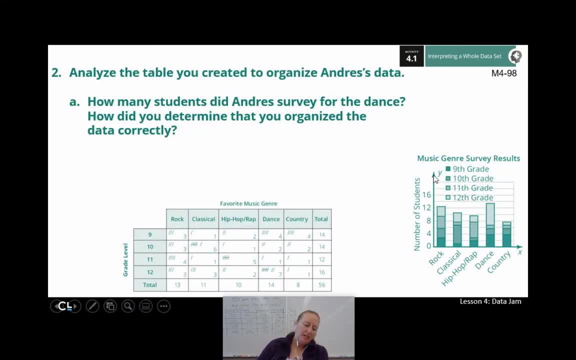 So can you just take a moment here to analyze on this data, right? So we have this table. We created and organized Andre's data. We also made a graph to go with it. Awesome, awesome, awesome. I have here on page one: I have a graph. 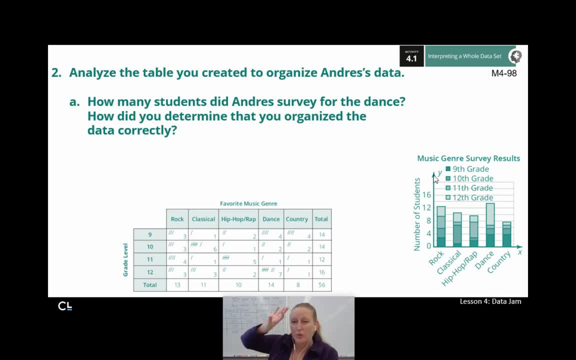 Here on page M4-98, I got four questions for you: A, B, C and D. Can you go ahead and take a look at your table, Take a look at your graph, And can you analyze this data and answer these lovely questions? 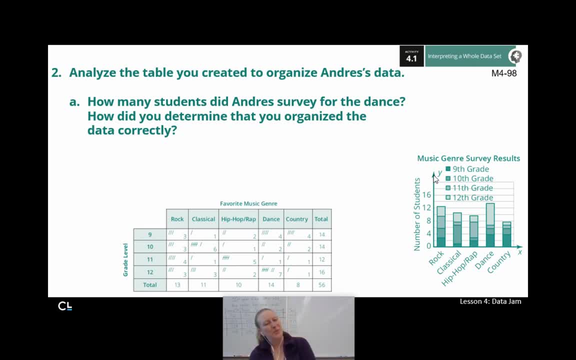 Go ahead, Hit pause, Answer the questions And hit play. when you're ready to check, Go ahead. So some of these are pretty easy to answer. How many students did Andre survey for the dance? We were looking at that earlier. He surveyed 56 students for the dance. 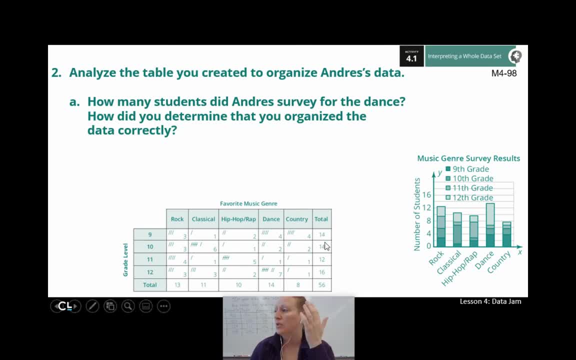 And I know that because if I add up these 14,, 14,, 12, and 16,, I get 56.. Or if I add up these 13,, 11,, 10,, 14, and 8, I get 56. 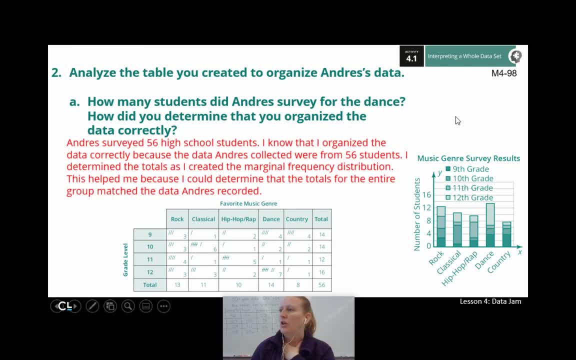 So we have a nice way of double checking our work there. So Andre surveyed 56 students. I know I did okay because my totals on both sides are adding up to that 56. So it just helps me make sure I add the things up okay. 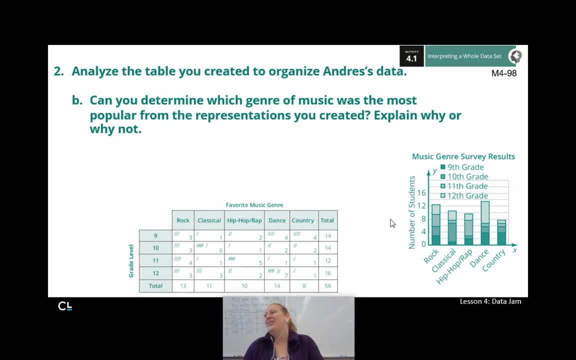 Can you determine which genre of music was the most popular from the representations you created? Yeah, As I look here, as I look here, I can definitely see what the preferences are. My dance bar is definitely the highest one, So I can totally see that dance is the most popular. 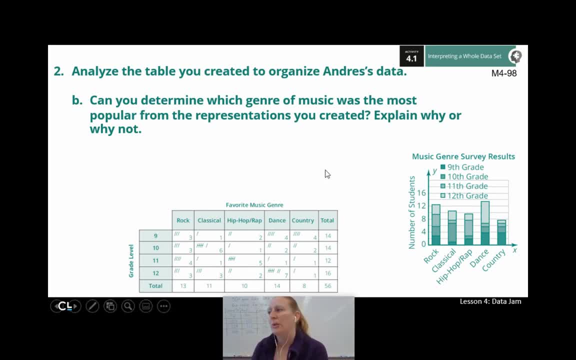 The country music bar is my shortest bar So it's my least popular. So I like the graph. I can totally see that country music was the least popular. I think it's preferred amongst the students surveyed And the most preferred was dance. 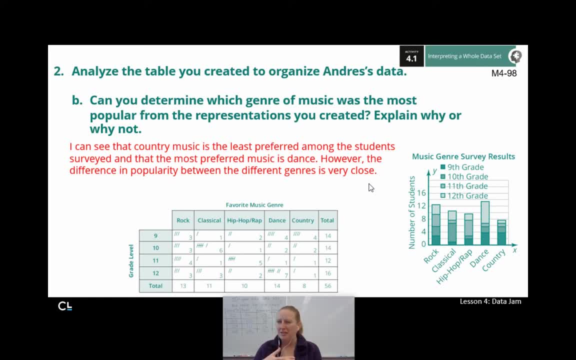 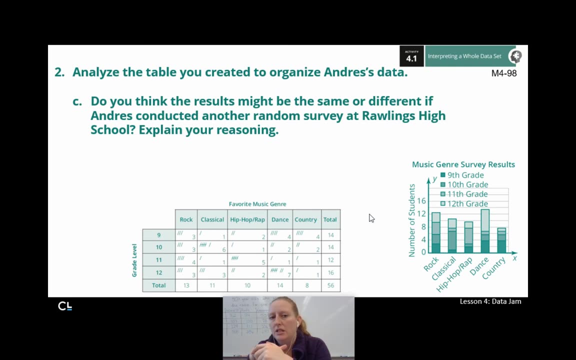 But for a lot of these the differences are pretty close. Like it's not extreme, right, I can see there's some These bars, some of these bars are really close. Do you think the results might be the same or different if Andre's conducted another? 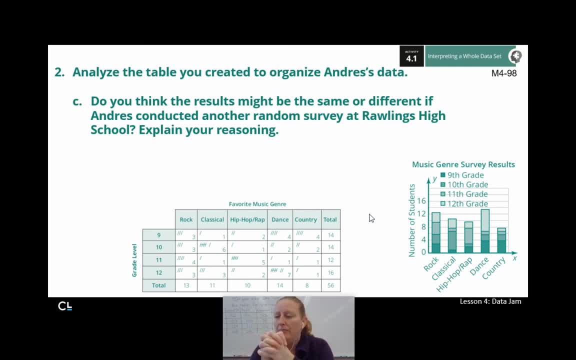 random survey at Raleigh High School. I think it could vary a little, right? I mean, we only have 56 students, So it's not like we're trying to get more students to respond. I suppose if we did things to try and get more students to respond, it could make the 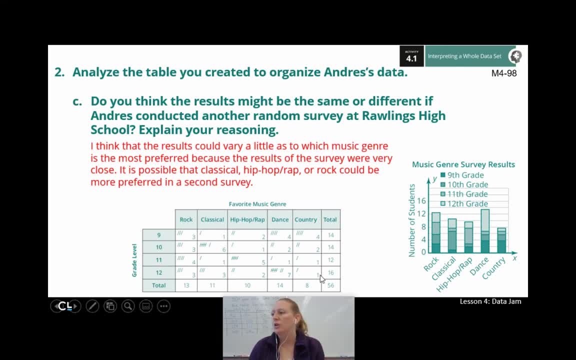 data vary a little bit, And I say that because these results were close right: 13,, 11,, 10,, 14,, 8.. These numbers are all pretty close. It's not like I got 20-something and then five right. 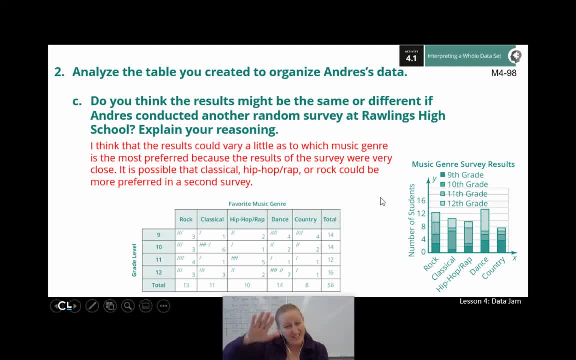 So I do think that another random survey might shift the data a little bit. It's possible that one of these others, like Rock, could overtake him and become the most popular. I don't know if it's going to be the second most popular here. 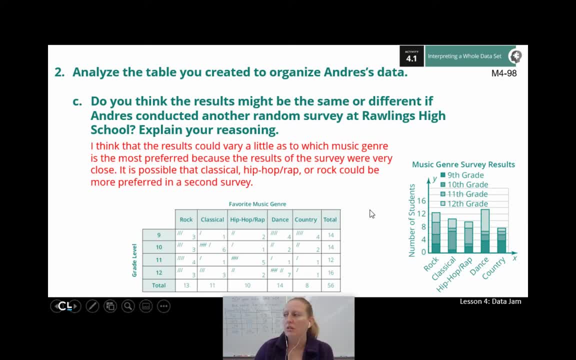 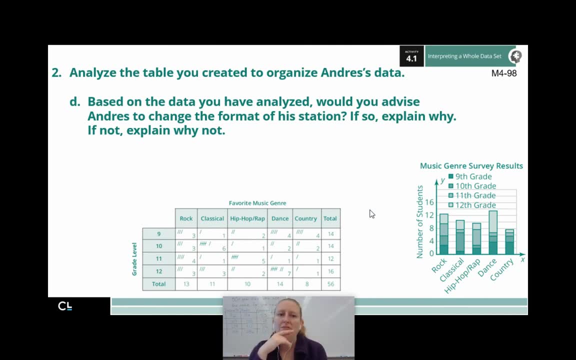 So different survey, It could vary, It could change our results a bit. Absolutely They're kind of close. So, based on the data you've analyzed, would you advise Andre's to change the format of his station And, if so, explain why? 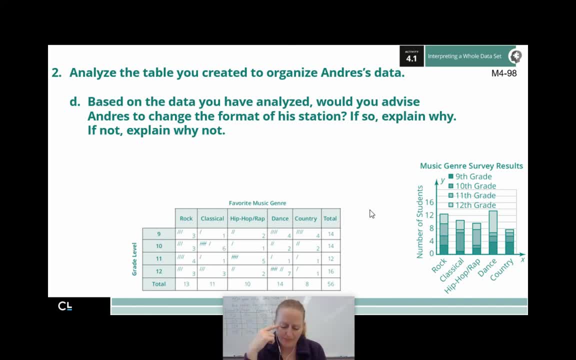 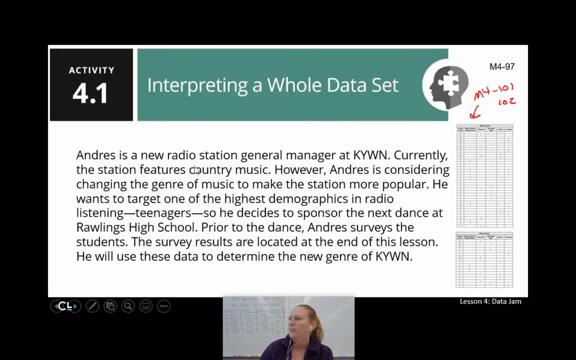 If not, explain why not. Well, I don't know, This one's a rough one, Like I was looking at it And hang on, I'm going to come back here. So real quick. So there is that. He and Andre are playing music.